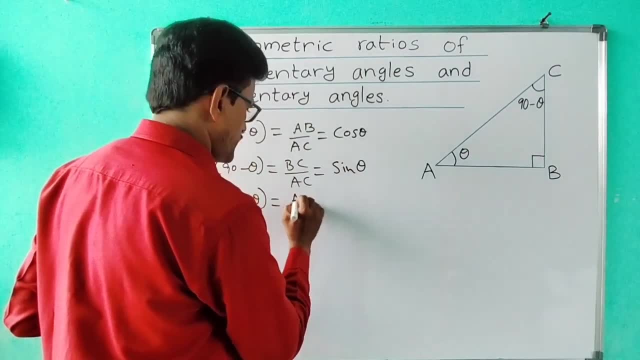 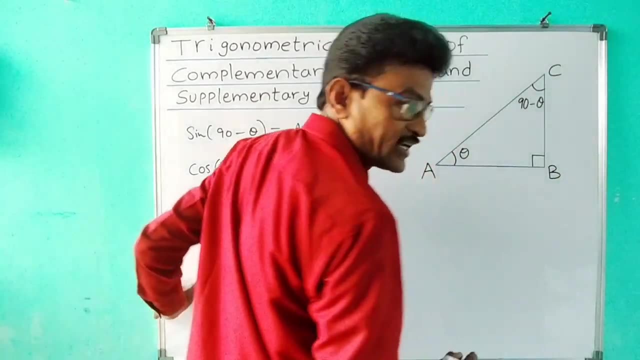 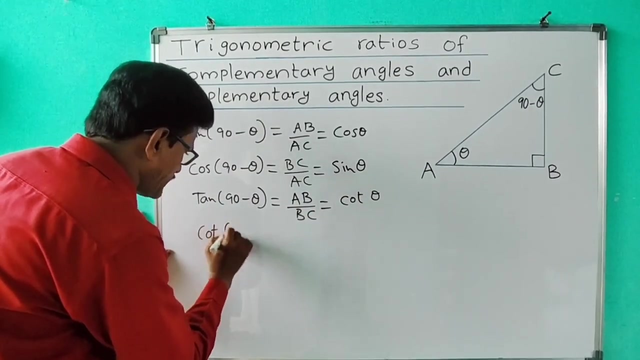 adjacent AB by BC. AB by BC Now with respect to theta, AB by BC. adjacent by opposite, it is cot theta, So tan 90 minus theta. we are getting cot theta Now cot 90 minus theta, So this is cot. 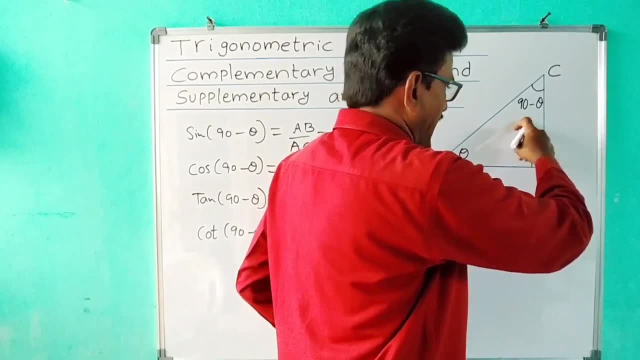 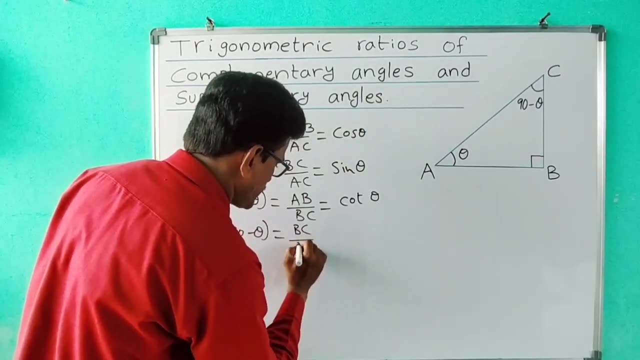 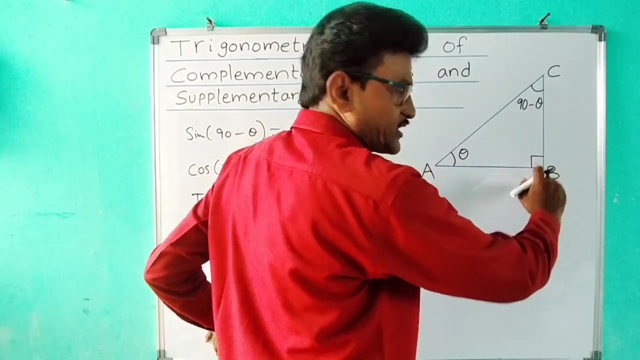 90 minus theta means this is 90 minus theta. So tan is opposite by adjacent, but cot is adjacent by opposite. So BC by AB, BC by AB, Adjacent by opposite, See with respect to theta. what is BC by AB Opposite by adjacent? So it is tan theta Opposite by adjacent means tan theta. So tan 90. 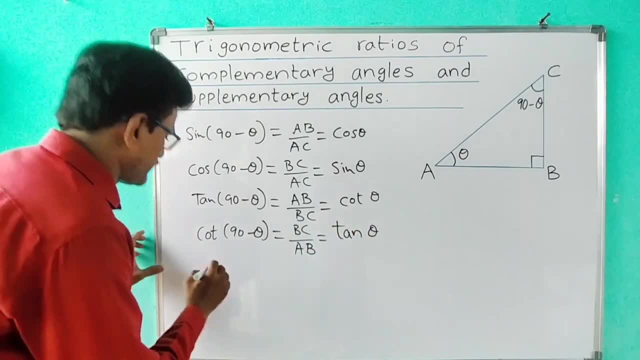 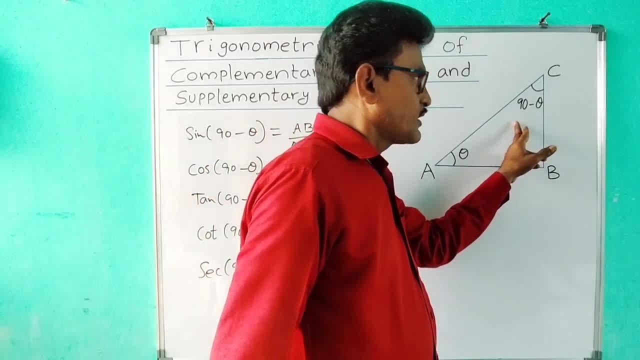 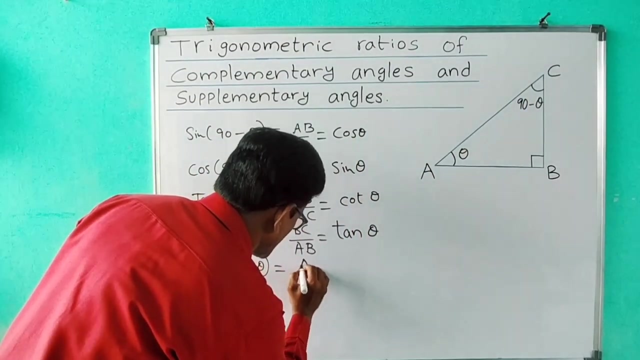 minus theta, we are getting cot Cot. 90 minus theta, we are getting tan theta. Now, what is 90 minus theta? Come here, Second: 90 minus theta. Cos means adjacent by hypotenuse. Second means hypotenuse by adjacent. So AC by BC, AC by BC. Now, with respect to theta, what is AC by BC, Hypotenuse? 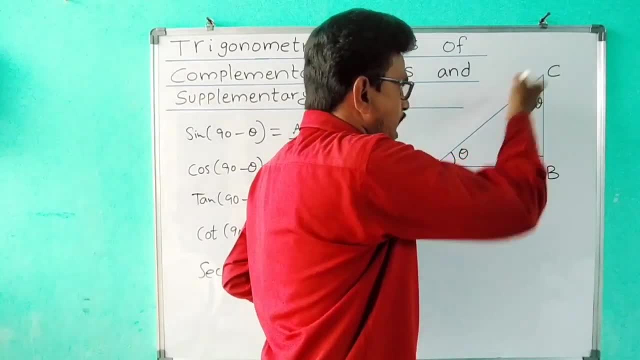 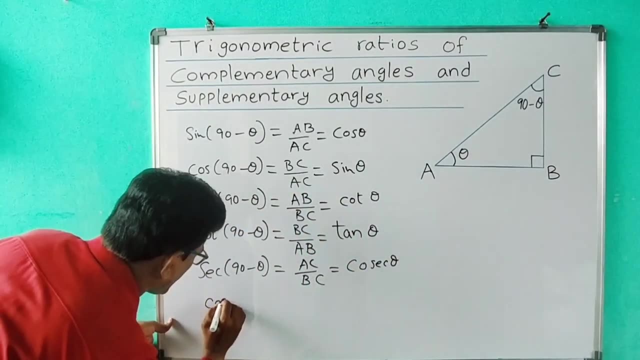 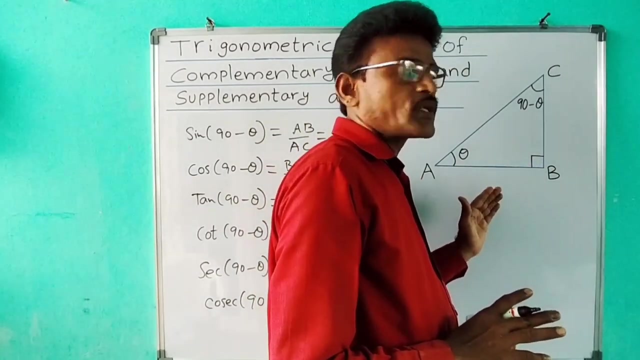 by opposite, Opposite by hypotenuse sine theta. So hypotenuse by opposite is cosecant theta, It is reciprocal cosecant theta. Now, what about cosecant 90 minus theta? is what? Cosecant 90 minus theta? It is reciprocal of sine theta. Sine means opposite by hypotenuse. 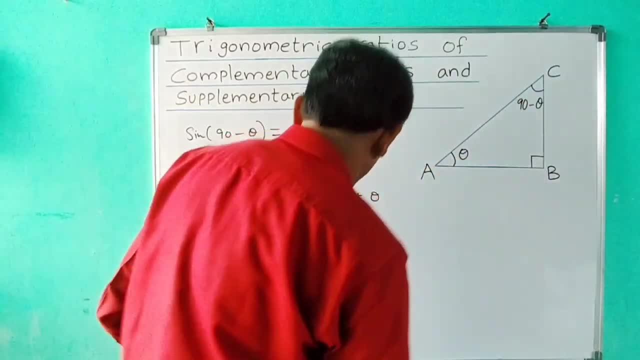 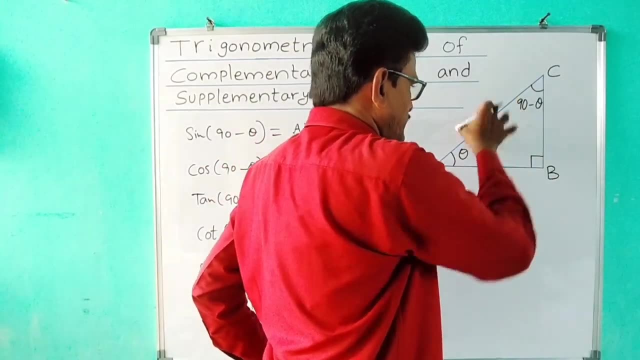 So cosecant means hypotenuse by opposite. So AC by AB, AC by AB. Now, with respect to theta, what is AC by AB? AC, It is hypotenuse, AB is adjacent, Adjacent by hypotenuse is cos. 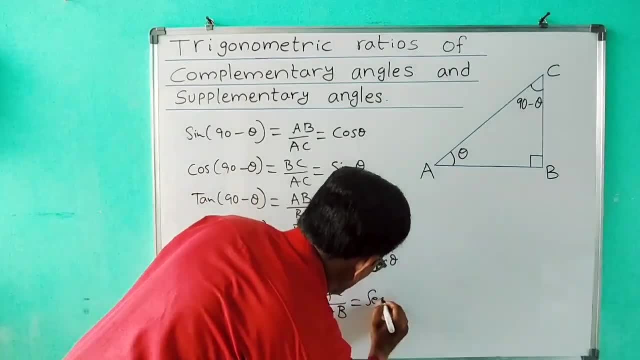 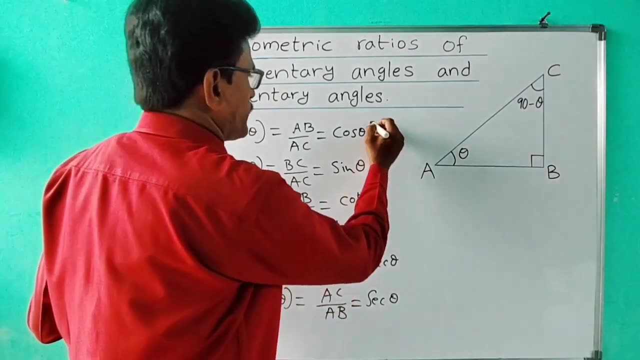 So hypotenuse by adjacent is secant theta, So secant is changed as cosecant, Cosecant changed as secant. So these two are cos Complement angles. Sine changes as cos, Cos will change as sine. Now tan and cot. So 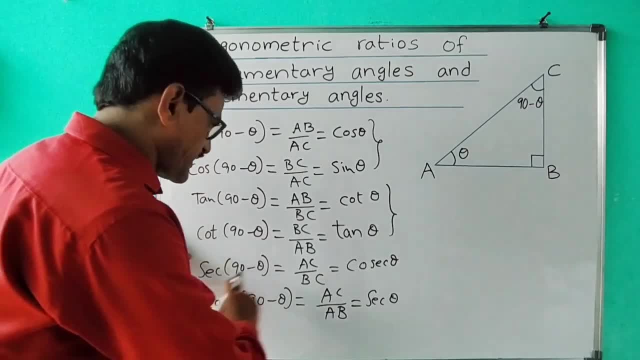 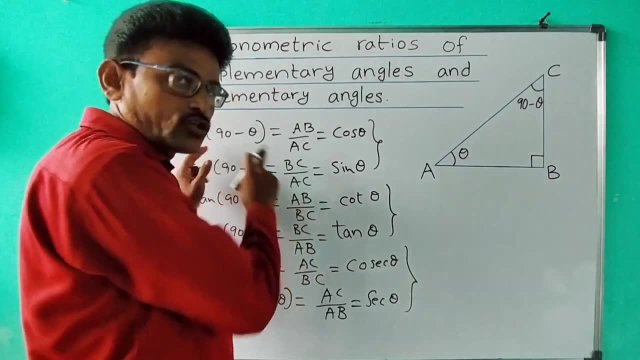 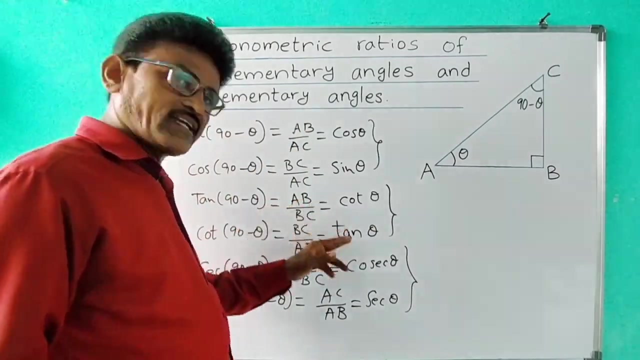 tan changes as cot, Cot will change as tan. Now, secant changes as cosecant, Cosecant will change as secant. These two are complement angles. So that's why sine 0 in trigonometric table, we are getting cos 90. Cos 0, we are getting sine 90. Like that, Tan 0, cot 90,. 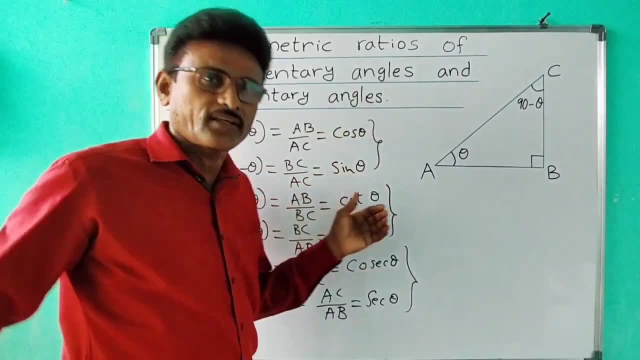 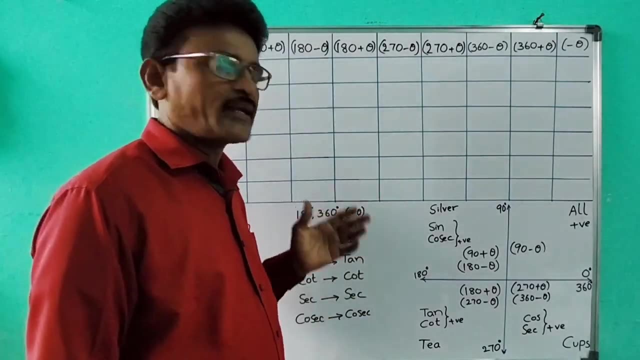 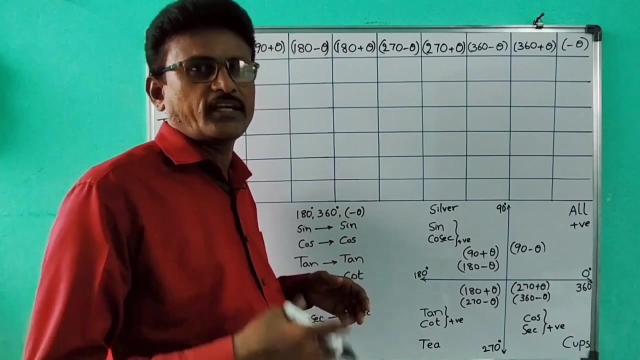 cot 90 table. we are writing in reverse order. These two are complement angles. Okay, Students, now I am going to fill total complement and supplement angles in this table. If you follow this table, this is useful not only in 10th class in the future PUC intermediate. 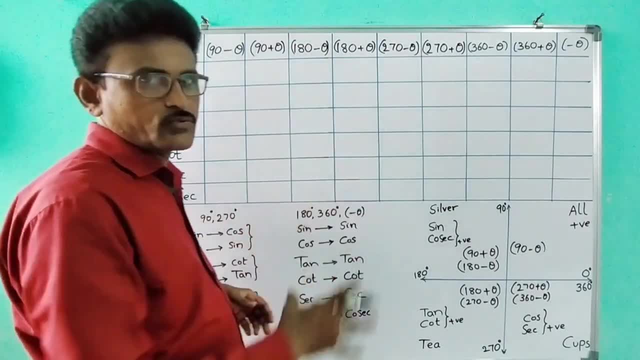 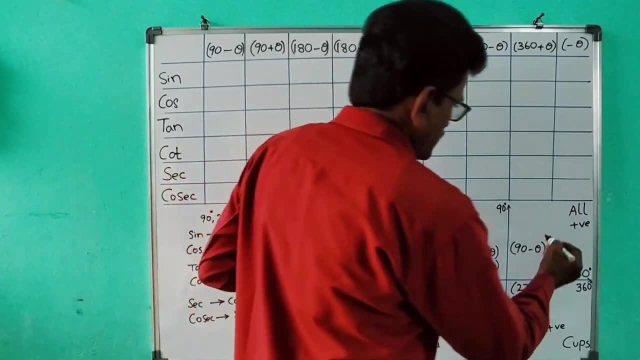 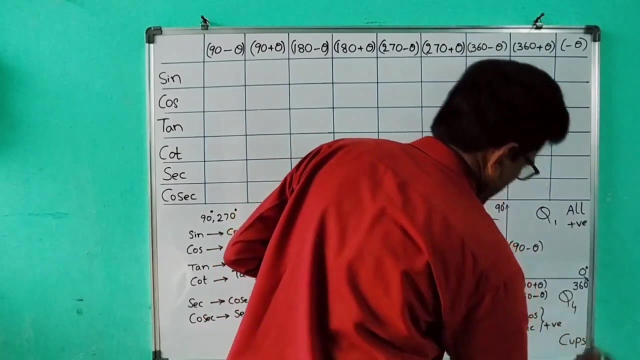 okay, diploma and for any completed exams. also, this table is very helpful. See this plane. I divided into four quadrants. Okay, This is quadrant 1, quadrant 2, this is third quadrant and this one is fourth quadrant. 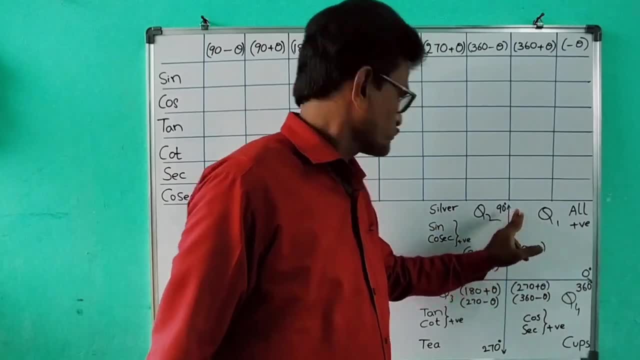 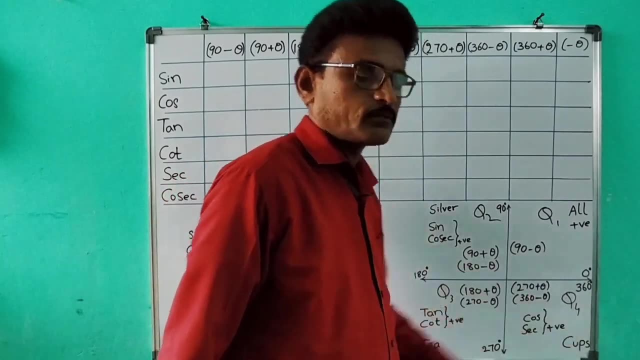 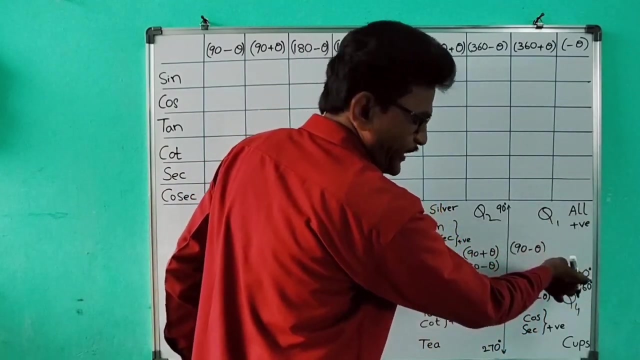 Okay, First quadrant, 0 to 90 degrees. Second, 9 to 180 degrees. Third one: 180 to 270.. Fourth quadrant: 270 to 360 degrees. Here in this quadrant, first quadrant, angles 90 or less than 90, 0 to 90. Okay, Means 90 minus theta lies in the first quadrant. 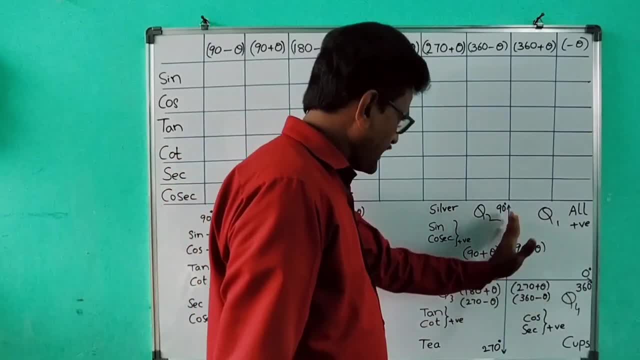 0 to 90.. Okay, 90 minus theta, 90 plus theta, it will be in the second quadrant. So when we write this particular line, we are getting cosine and sine and cosecant, and these two are complementary angles. So total complement angles are 0 and 90, here. So we are getting 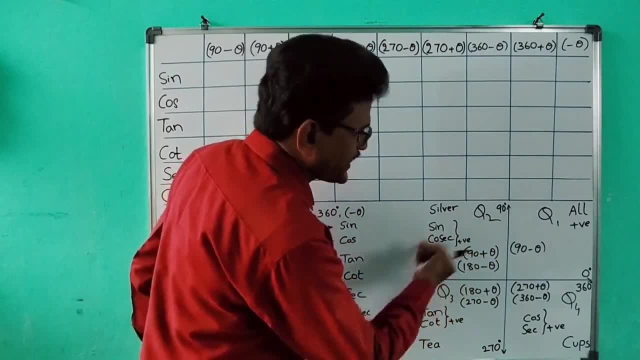 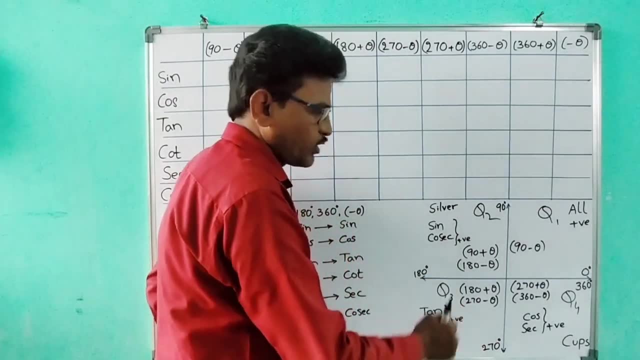 cosine sine and subcontractive angles: Okay. So when we are writing this product, this okay, 180 minus theta- also in second quadrant. 180 plus theta in third quadrant. 270 minus theta- also third quadrant. if angle is 270 plus theta, it is fourth quadrant. 360 minus, also fourth quadrant. 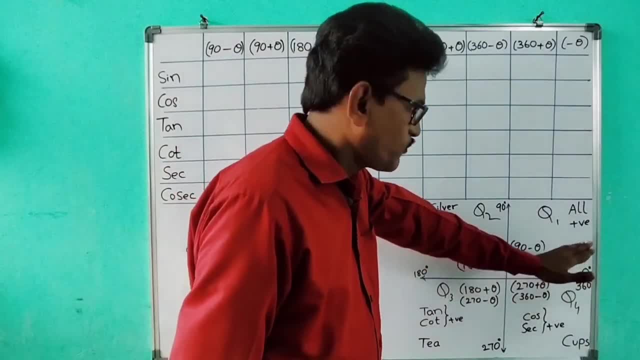 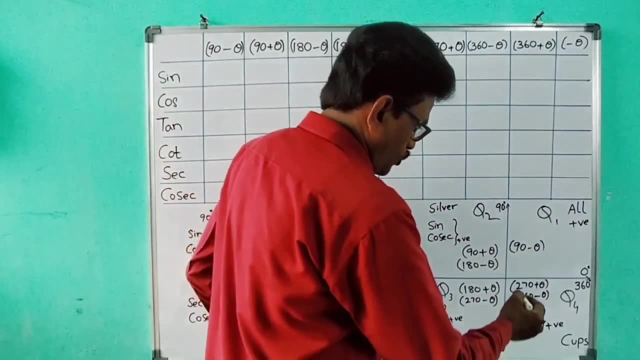 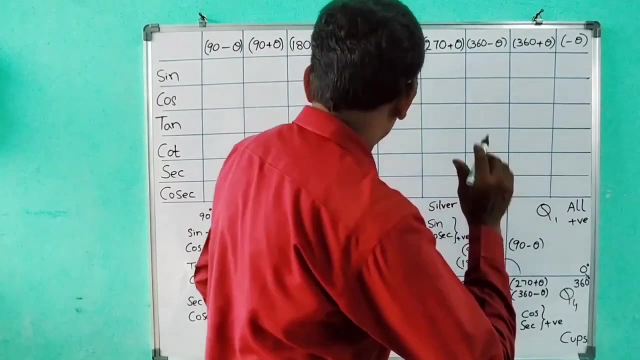 once again: 360 plus means you will go to first quadrant, minus theta means you will come back. okay, fourth quadrant, like that. so always, actually, we will take theta in anti-clockwise direction will be positive. if you move clockwise direction, angle will be negative. okay, now we will discuss. 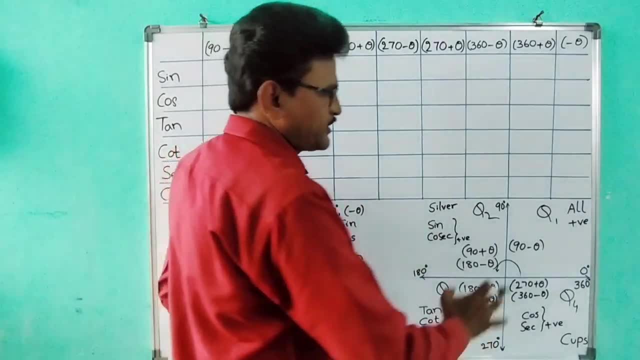 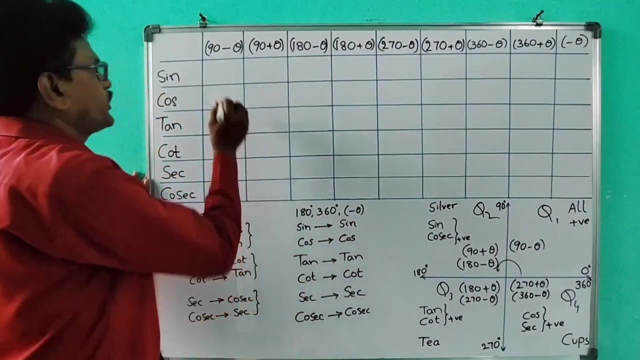 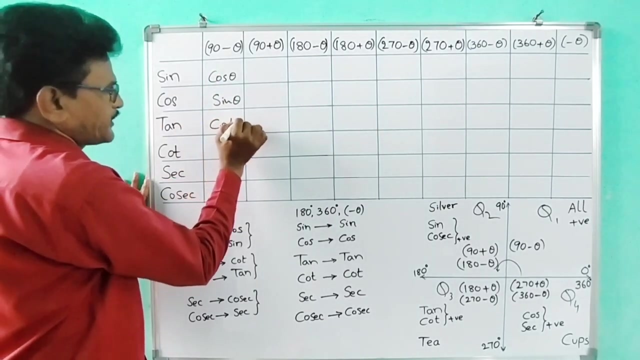 about first quadrant already just now i explained: sine 90 minus theta, cos 90 minus theta, all will fall in first quadrant sine 90 minus theta, when it is cos theta, cos 90 minus theta, sine theta, tan 90 minus cot theta, cot 90 minus theta, tan theta. okay, sine will change as cos cos will change? 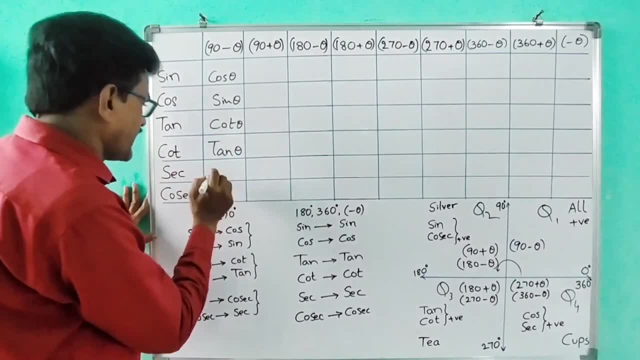 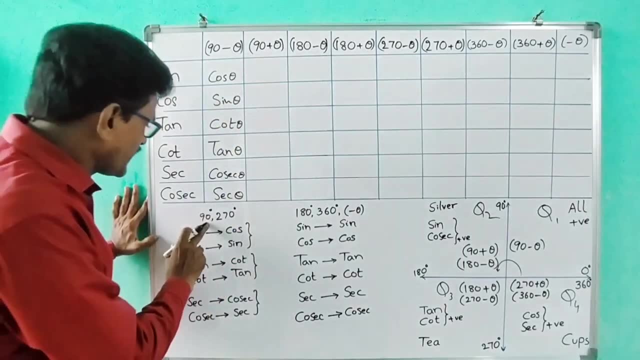 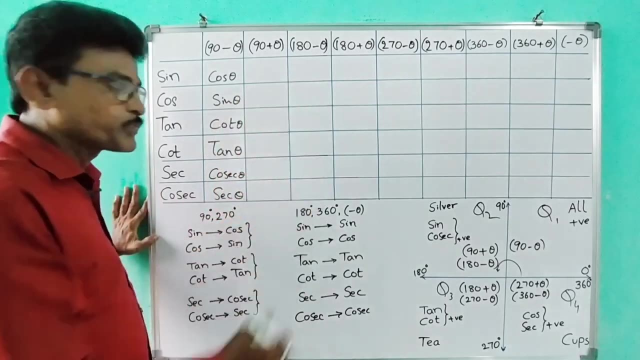 as sine. tan will be cot. cot will be tan. next secant. secant will change as cosecant theta, cosecant will change as secant theta. i explained already similarly for 90 sign changing cos like the 270 degrees also sign will change as cos. cos will change as sign. okay, now for 180 degrees and 360 degrees, sign will be sign. 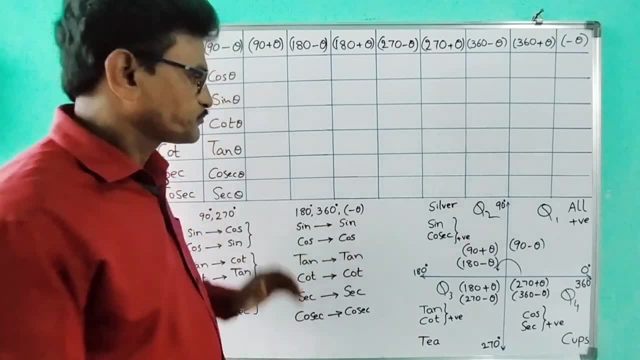 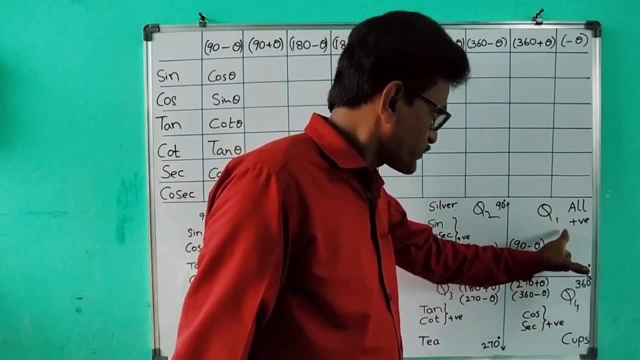 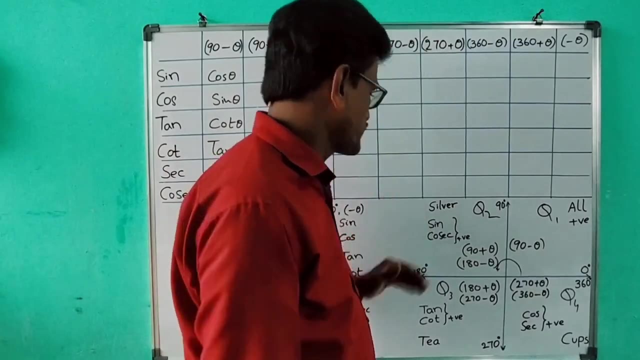 cos will be cos, tan will be tan, cot will be cot, like that. and one more thing, why we are telling here: all means in this quadrant all are positive. okay, all are positive means. that's why here we entered: all are positive values. now, what about second quadrant c, for remembering purpose all? 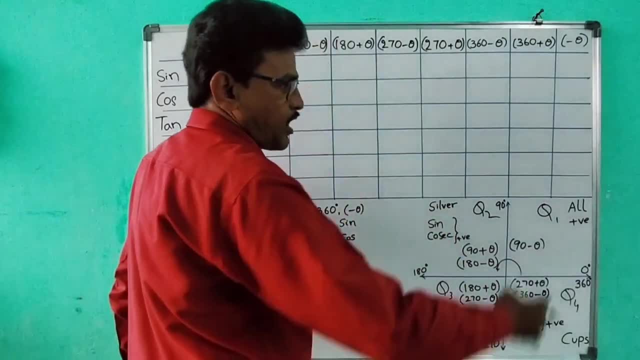 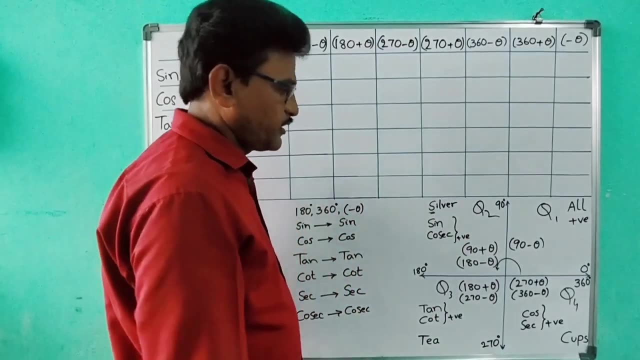 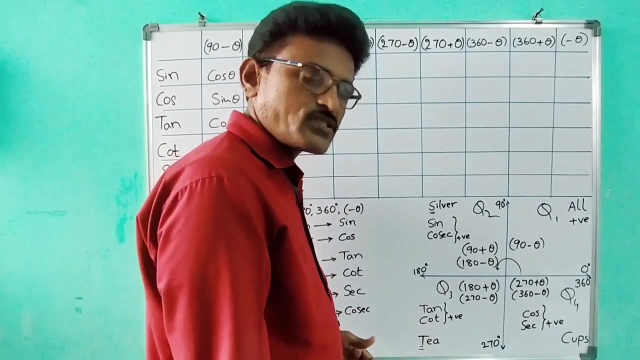 silver tea cups. i enter like that. it means what all are positive. see here: first letter is yes. it means sign and cosecant positive. remaining four negative in this t. first letter is t. it means negative, tan and cot positive and other items negative in this cups. first letter is c. so cos and secant are 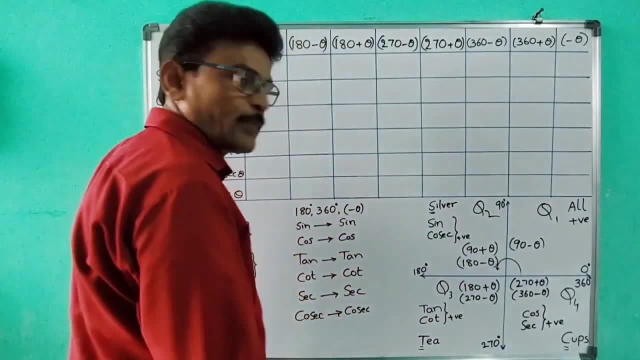 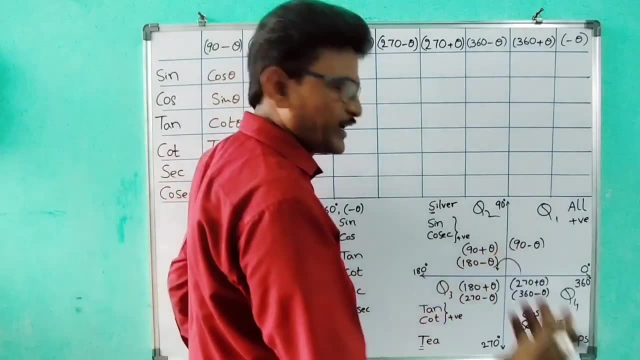 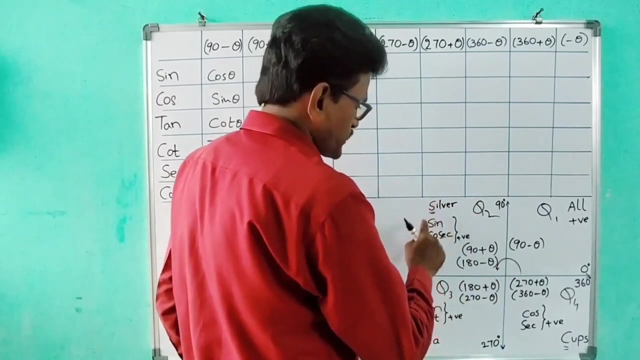 positive, other four negative. so for remembering purpose, we are writing all silver tea cups with first letter. you can remember that which is positive and which is negative. somebody will remember. like this: all students take coffee. like that also. okay, students means. first letter is sign cosecant. okay, all students take. 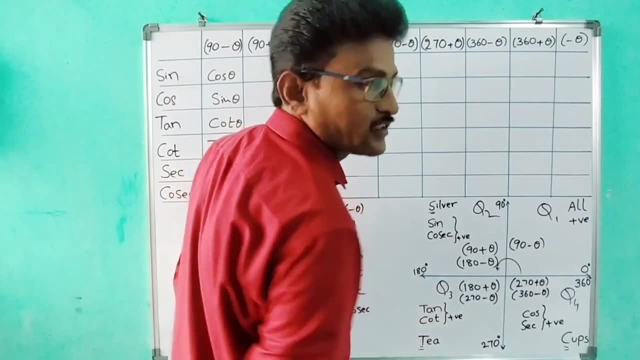 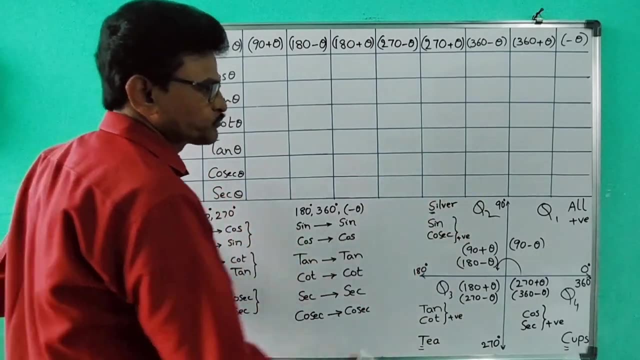 coffee and a coffee led by c, tan and cot. first letter is c, cause and secant. because we can remember anyway. now i am going to complete 90 plus theta in this second quadrant sign and cosecant values. use positive sign and also cosecant, these two. 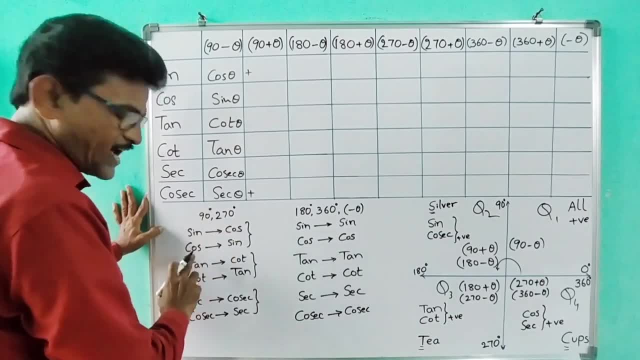 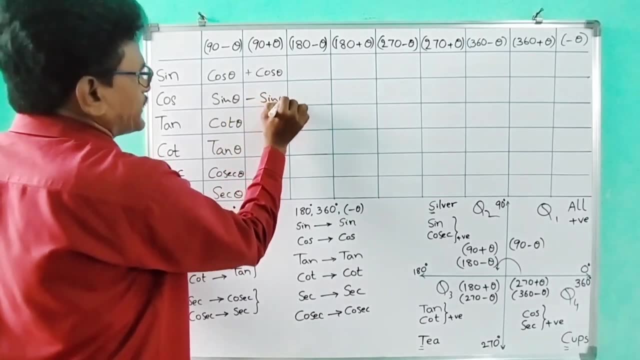 positive and also what i tell: sign will change as cos cos will be sign. so sign will change as cos remaining items negative. cos will be sictheta, tan will be cot negative. and this the road is. the road will be습니까, say I know the next chapter is that the next chapter will discuss. 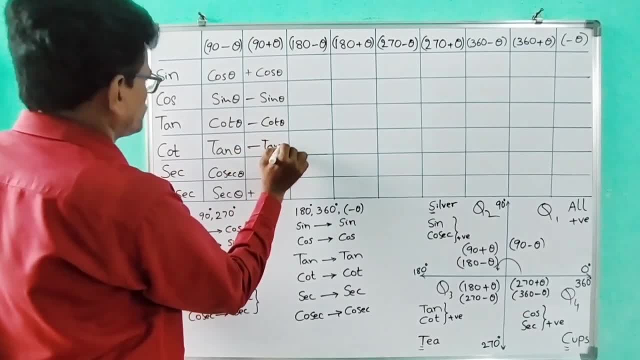 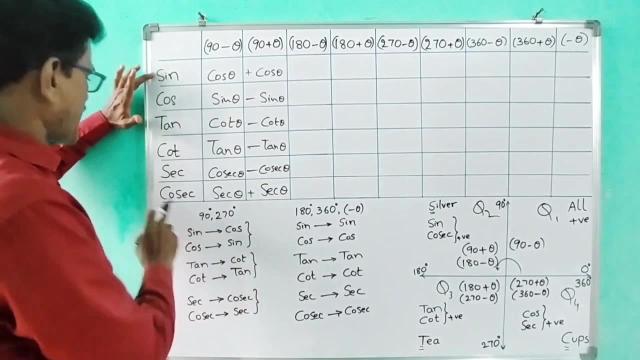 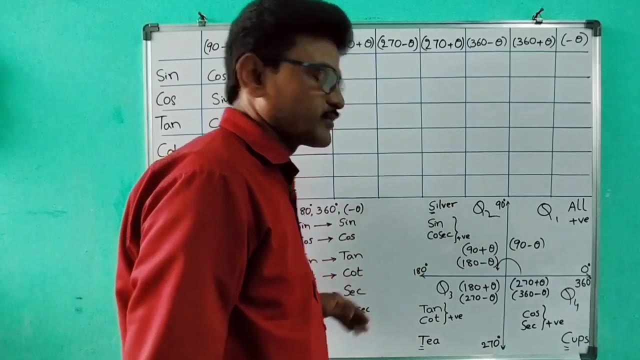 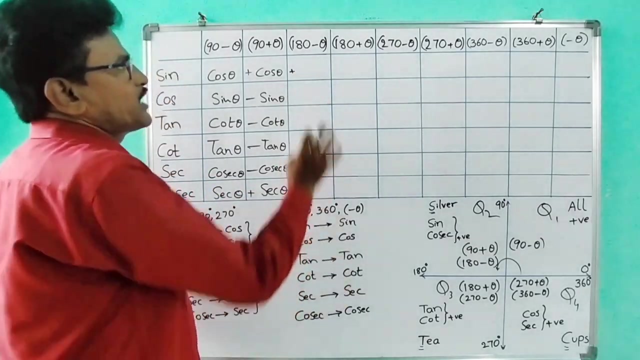 negative cot will be tan negative now secant, also cosecant, negative, now cosecant and secant past. so only sine and cosecant values, past two in second quadrant. now what about 180 minus theta? it is also second quadrant. it means once again here sine and also cosecant past two remaining for negative and 180 and 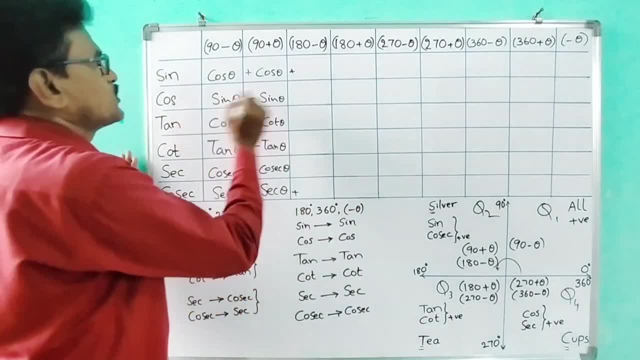 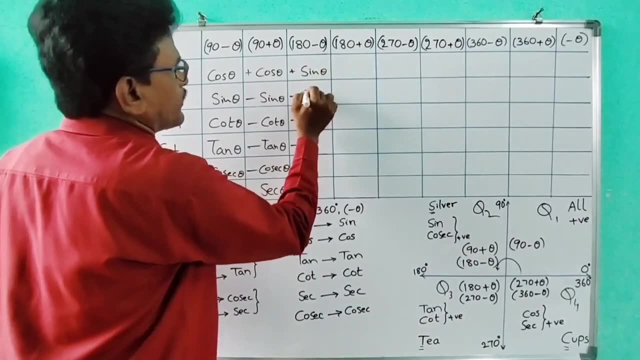 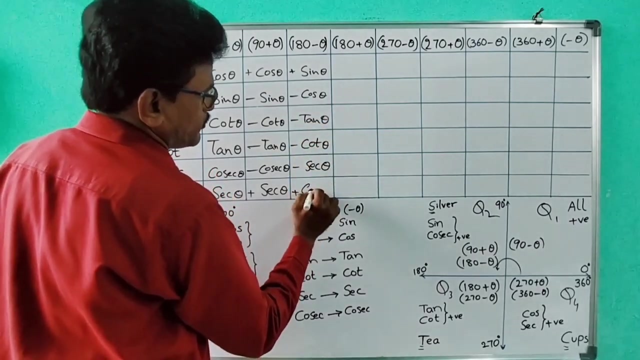 360, I told you sine sine cos cos, as it is what I write. so remaining four you can write as negative symbol: sine sine, only sine theta cos. theta, tan theta, cot theta, secant theta, next, cosecant theta, like that. now, what about 180 plus? it is third. 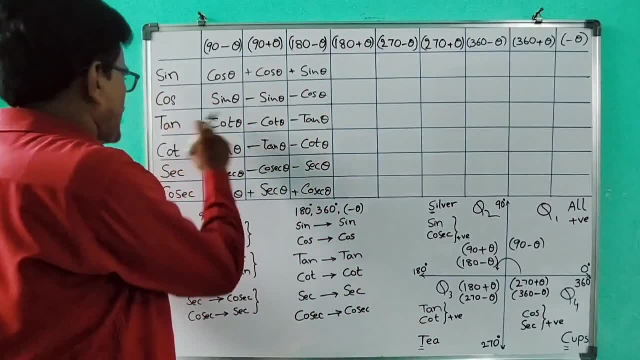 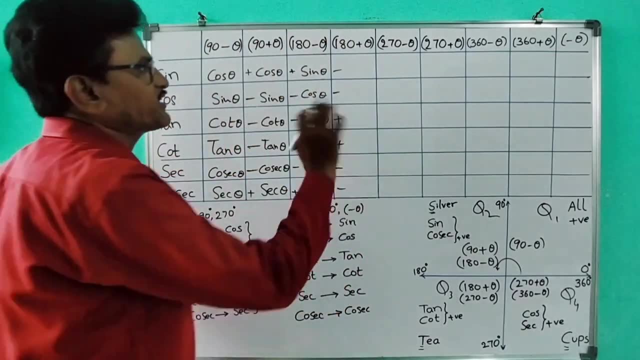 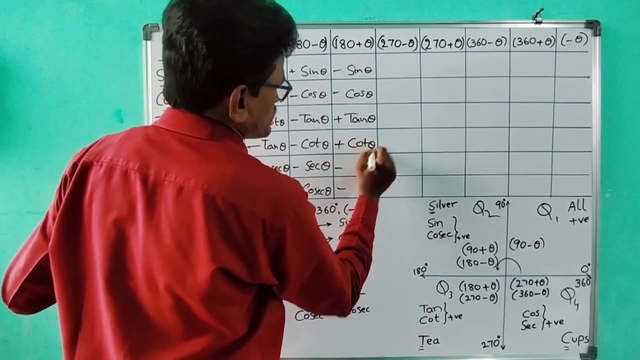 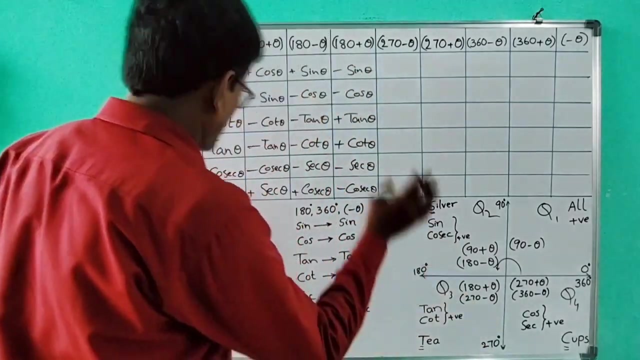 quadrant. in third quadrant, tan and cot positive, see tan and cot, these two positive, remaining for negative. and 180 means as this sign: sign cos, cos. now we can complete: sign cos tan, cot, secant, cosecant, like that. okay, now 270 minus. it is also in third quarter. in third quarter, once again tan. 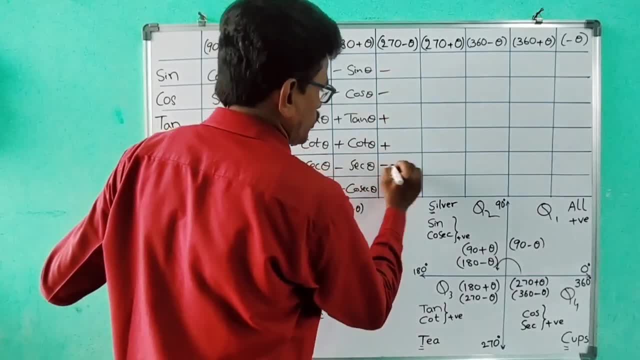 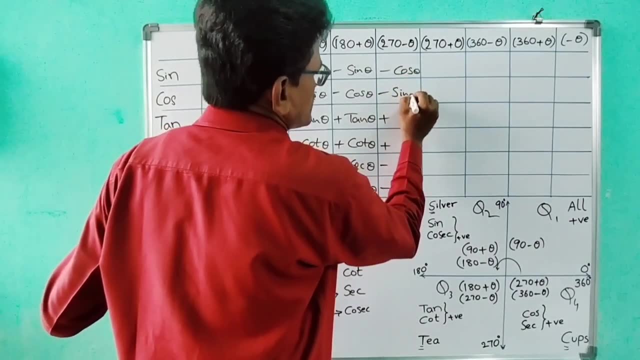 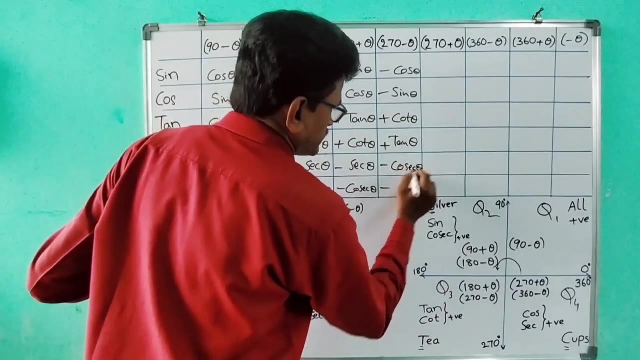 and cot positive, remaining for negative. so 270 means change sign as cos cos as sign. sign will change as cos cos will change as sign: tan will be cot theta, cot will be tan theta, secant. it is cosecant, then cosecant will be secant like that now. 270 plus, it is fourth quadrant. 270 plus means: 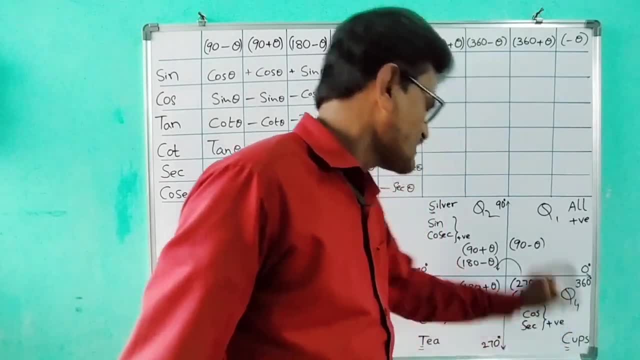 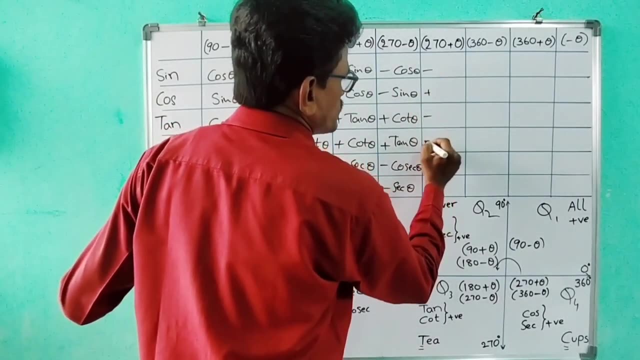 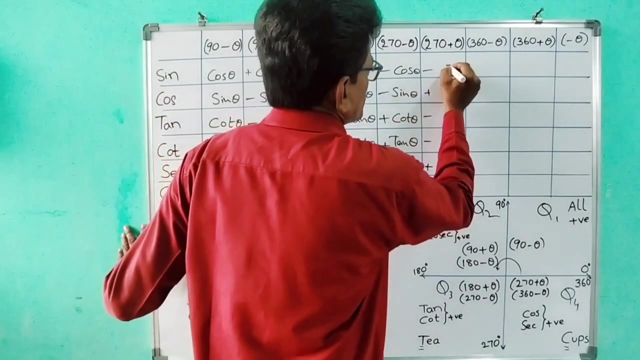 you entered into fourth quadrant. in this fourth quadrant, cos and secant positive, see cos positive and also secant positive. remaining for negative symbols: 270. once again, 270 means sign, sign. sign will be cos, cos will be sign. so sign will be cos. theta cos will be sin, theta tan will. 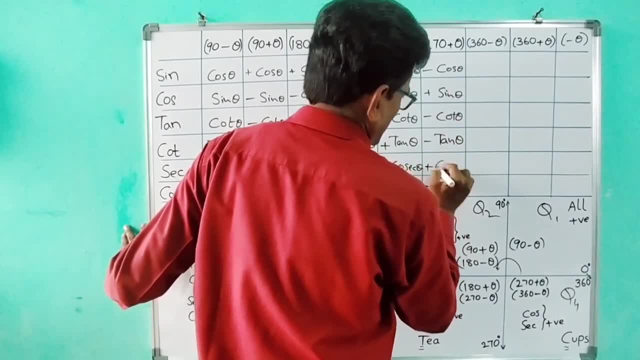 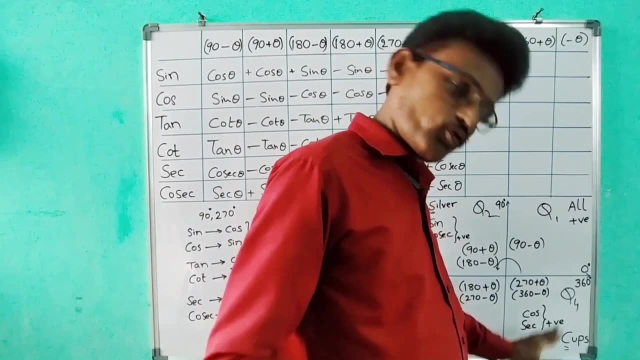 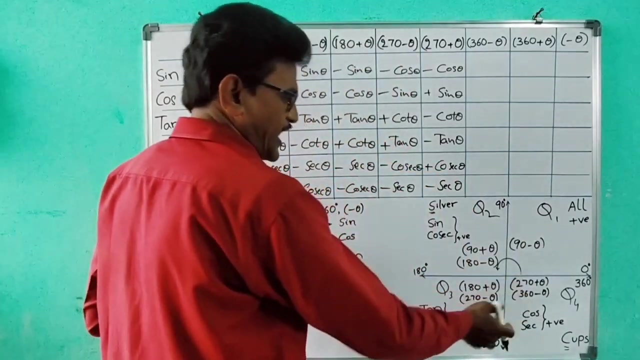 be cot cot changes tan theta. secant changes cosecant theta, cosecant changes secant theta. finish now. 360 minus same fourth part, and only here. you have to remember: 360 means sine sine cos, cos. and also one more thing: cos and secant positive. okay, cos item and also secant item. 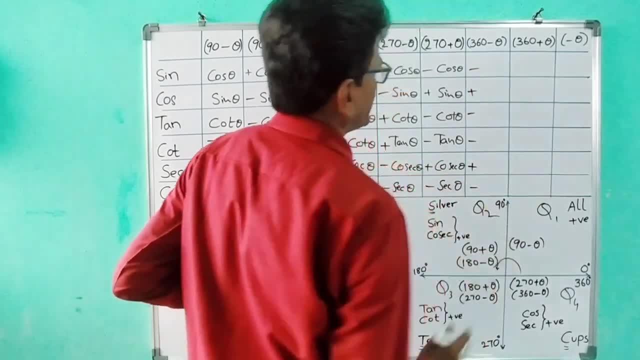 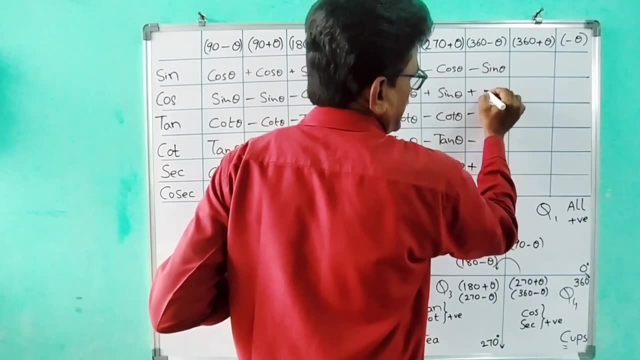 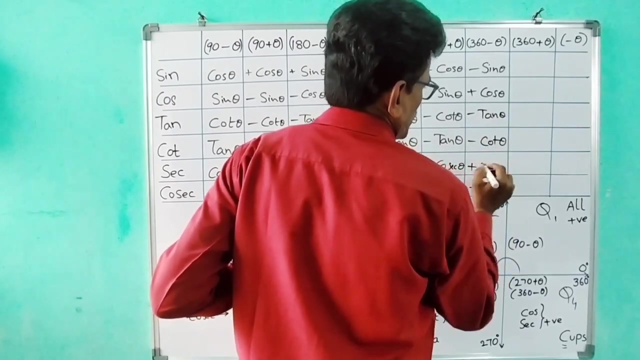 positive, remaining four negative. okay, so say sine 360, minus theta, sine theta, but minus symbol: cos 360, minus cos theta, tan 360 minus theta, minus tan theta, like that, this is minus cot theta, this one is my plus secant theta and minus cosecant theta. now 360 plus you entered into. 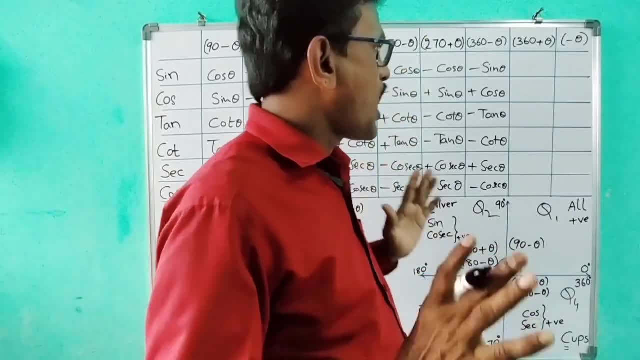 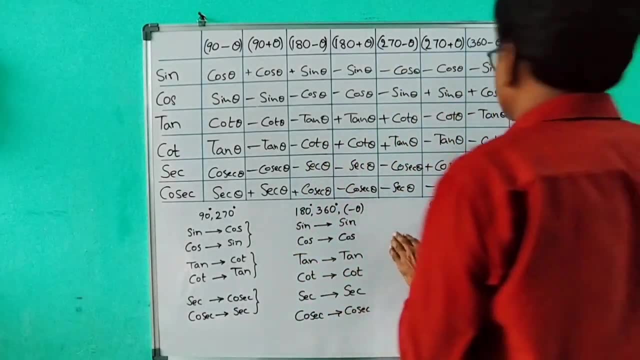 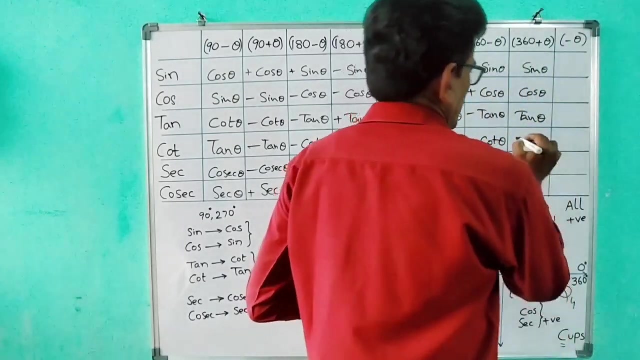 first quadrant. okay, in this first quadrant we know all are positive symbols only. so sign, sign only. 360 means i told you already sign, sign, cos, cos like that. so here you can write us sine theta, cos theta, tan theta, next cot theta, secant theta and also cosecant theta, so as this: 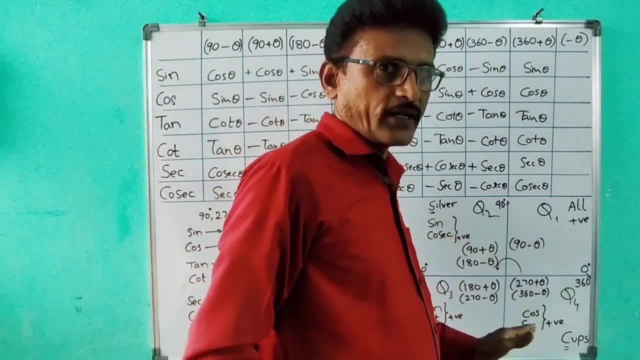 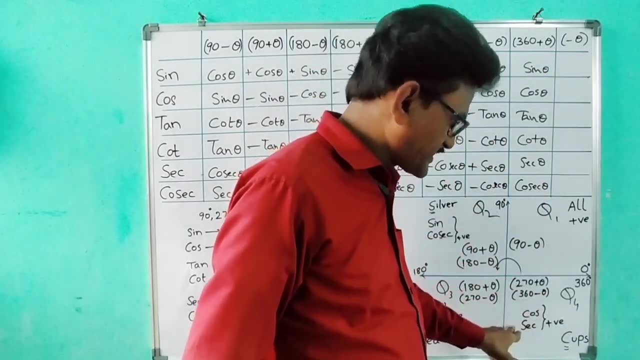 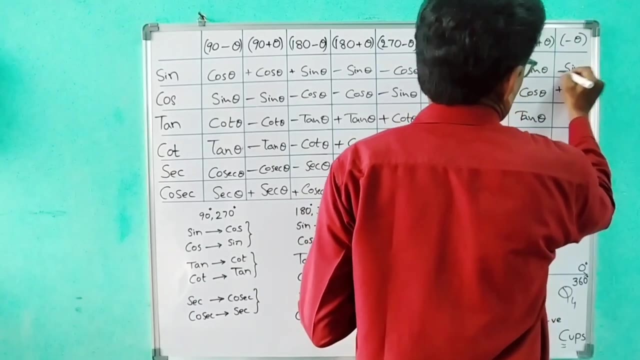 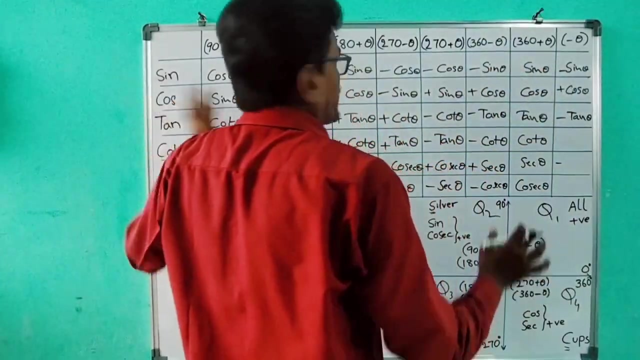 we have to enter 360 plus. it means first quadrant, next minus theta, sine minus theta. minus theta means here fourth quadrant cos and secant only positive so cos and secant positive sine sign only, but minus symbol cos, plus cos theta tan, minus tan theta. it means sine half minus theta, minus sine theta, cos of minus theta, cos theta tan half nice. 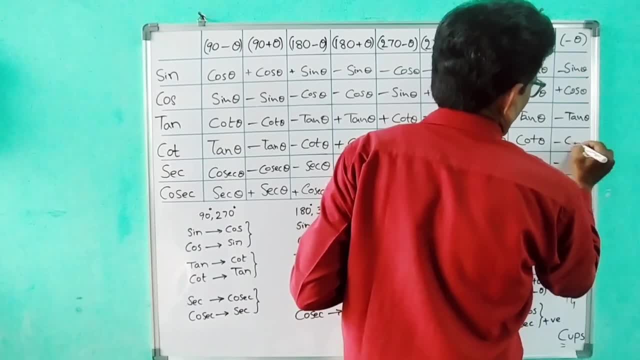 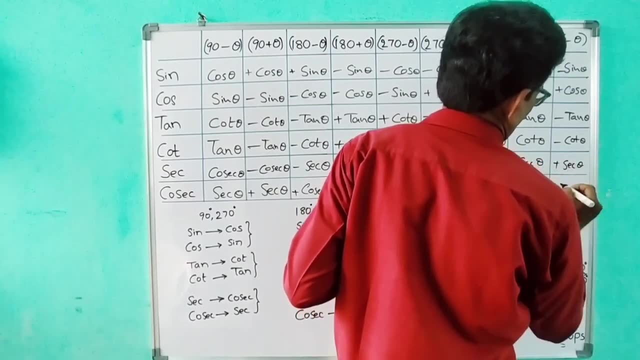 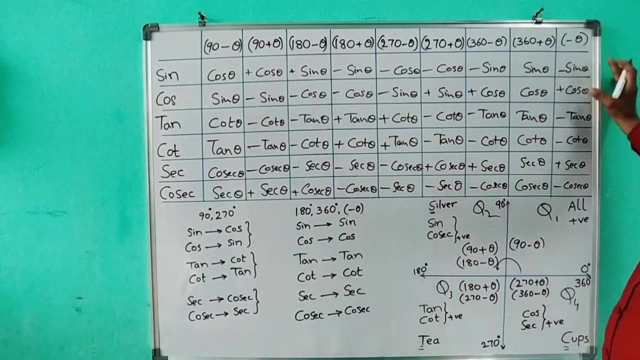 tita minus, then tita cot of minus tita minus cot tita. next, secant secant will be plus symbol. okay, plus secant theta. cosecant will be minus cosecant theta. so Remember when minus theta means cos and secant only positive symbols. 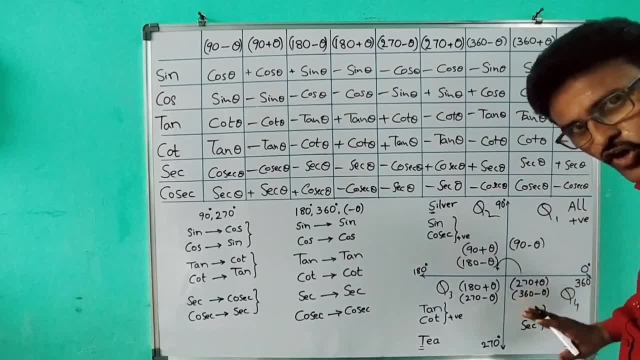 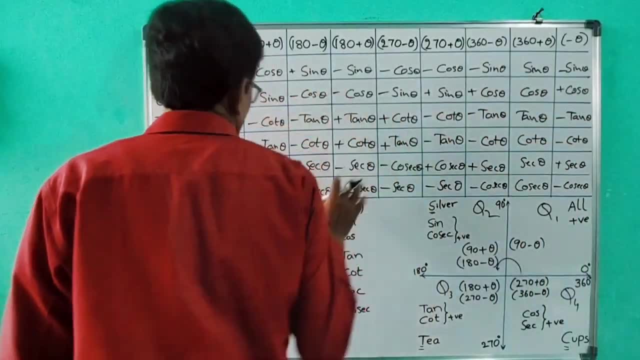 Because see, minus theta means you are coming into 4th quadrant Here, cos and secant, only positive. Okay, See, like this we can fill all these things Right. In the next video on this table we will solve some problems. 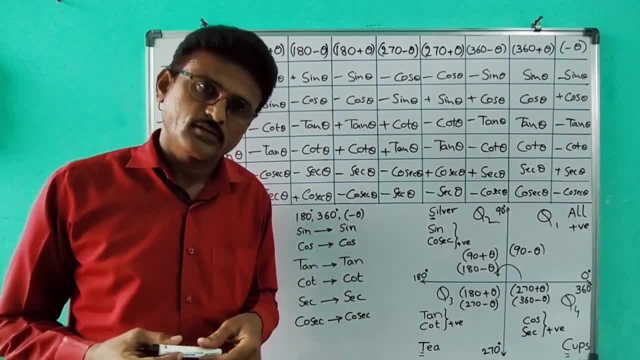 If you like my videos, please share, comment and subscribe my channel. Thank you.